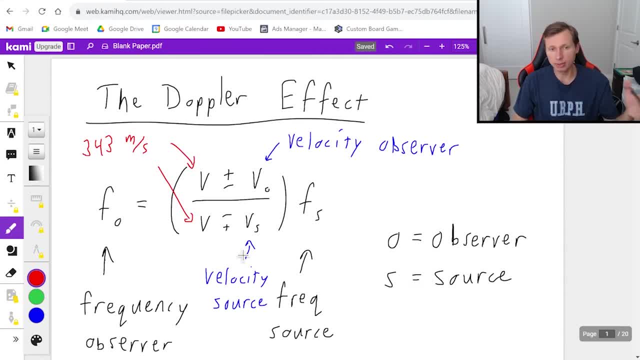 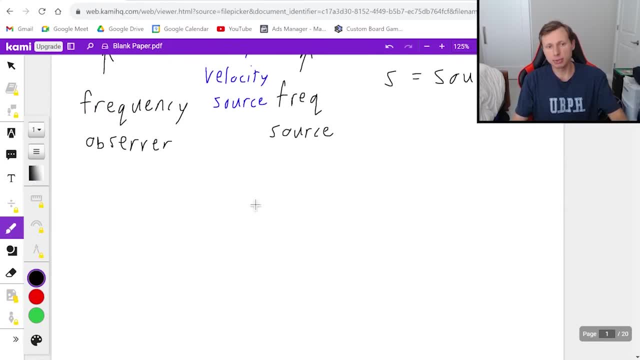 speed of sound in air. so, for instance, a siren blaring its horns and you hear it. that would be an example where you use 343 because it's the speed of sound in air. in other examples you might use v, equals three times ten to the eighth meters per second, which is the speed of light, but you would only be using this. 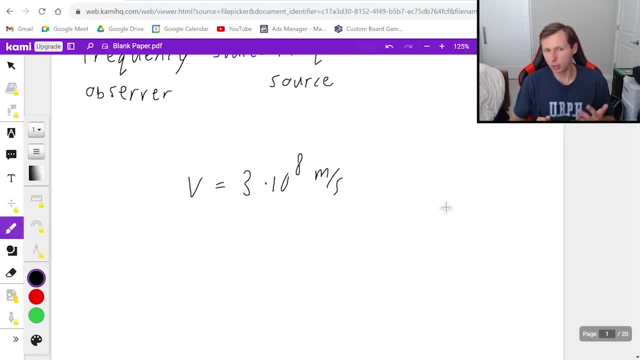 if we were talking about doppler effect for an electromagnetic wave, which is how doppler radar works. but if you don't understand that, i'm probably going to cover it in another video. so let's just focus on speed of sound in air for today, which is the 343 meters per second and the 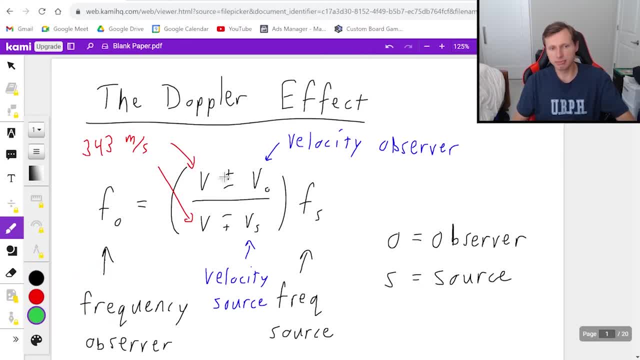 last thing to explain is the minus plus and the plus minus. very strange. it's probably the only equation that i know of that has a minus plus in it. here's what i would say for the pluses and the minuses: we're going to use the top whenever the object is heading toward you, and you're going to 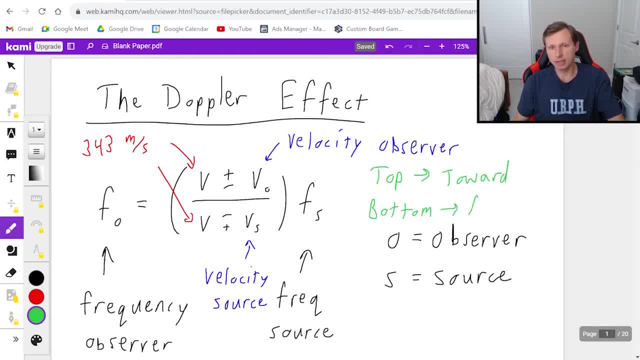 use the bottom sign, whether it's plus or minus, if the object is heading away from you. now, by the way, it is possible for both to be toward, both to be away. you can have one of each, one toward, one away. you can also have one is toward and the other is zero and it doesn't. 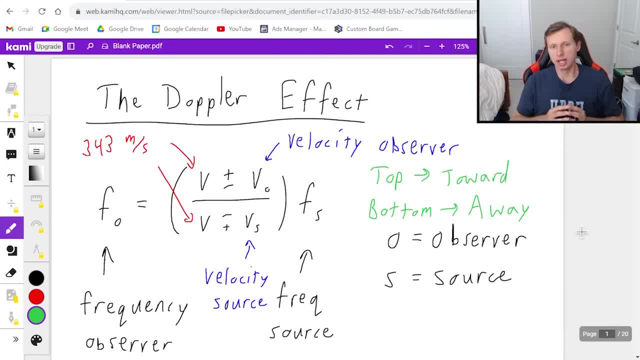 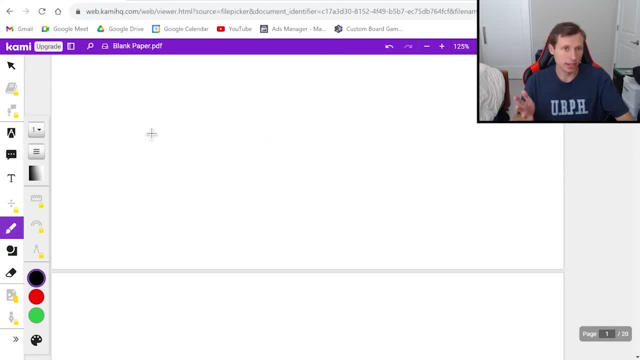 matter if it's plus or minus, because plus or minus zero is the same thing. and if you don't understand how that's possible, don't worry. we have a couple examples today that will make sense of it. so now let's look at a couple examples. number one: let's say a car is heading towards you with a velocity. 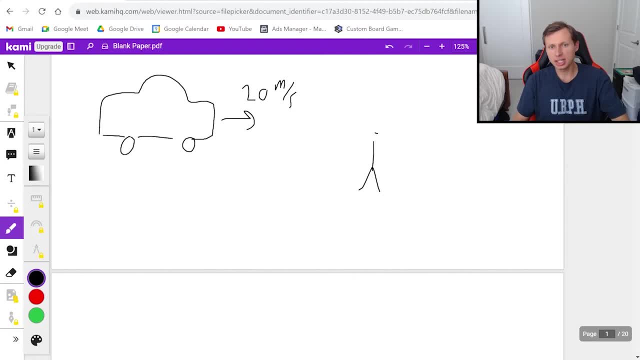 of 20 meters per second. you are standing here, you're not moving, and you are at rest here. your velocity is zero and let's say the car's horn has a frequency of one thousand hertz. that's the actual frequency of the car. but the question i'm going to ask is: what frequency do you hear? 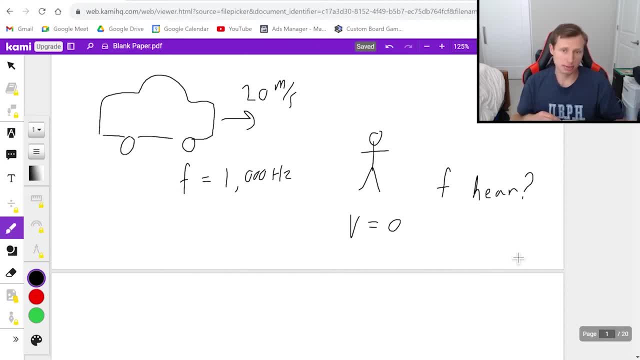 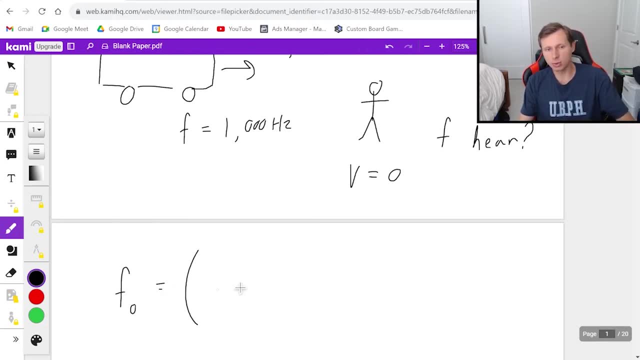 that's my question. so to do that, you're the observer and so we're just going to plug into the doppler effect equation with that happyную. the numbers we have. Frequency of the observer equals, the velocity is 343, and then I have to think: is it plus or minus? and that is a trick question. The reason why is because, even though 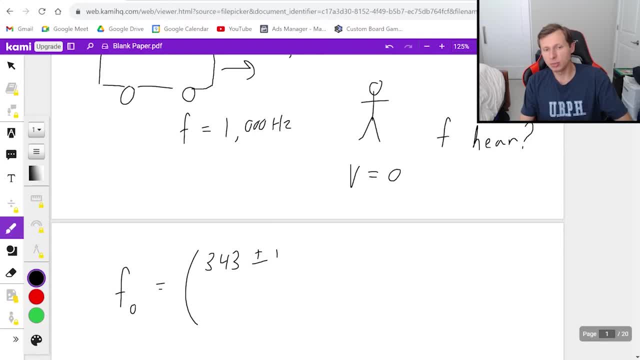 the car is heading towards you and it should be the top. the problem is in the numerator is the observer and you, the observer, are not moving, so it's plus or minus zero, which again it doesn't matter. if it's plus or minus zero, it's still just zero. What matters for the top and the bottom is: 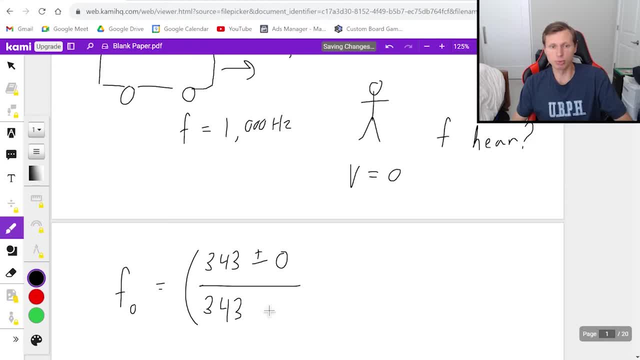 the denominator, because that has the source. The source is moving towards you. I use the top, which is minus, for the denominator. if you don't believe me, check the equation. and that speed of the car is 20, which goes right there, and then finally times the frequency of the source, which is 1000. 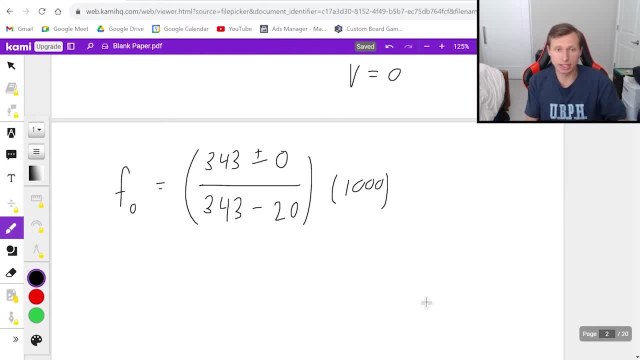 and you can just plug this in a calculator and we'll get our final answer. It looks like we're going to get a frequency of about 1062 hertz, which makes perfect sense because, in general, whenever the object is heading towards you, it means that the frequency is going to be a little bit louder than 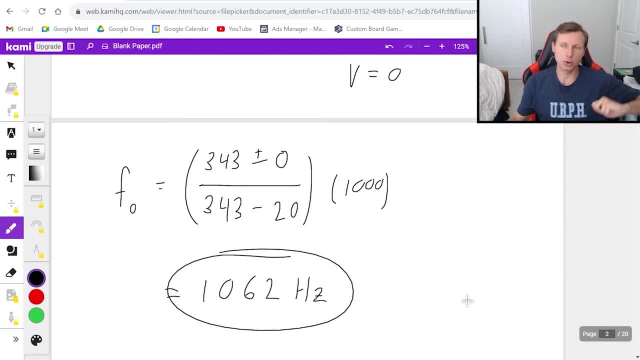 normal, and whenever it's heading away from you, it should be getting quieter overall. Now here is the next problem. this one's going to be a challenging one. Let's say you're running away from a bear and you know bears are scary because they're pretty deadly, so let's make this bear as angry. 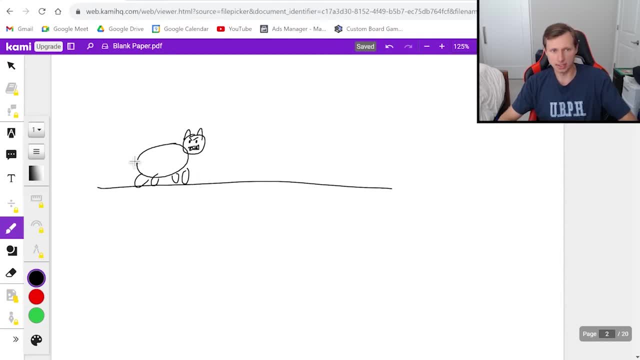 as possible. Yep, no, that's an angry bear, if I've ever seen one. Do bears have tails? Okay, this one will. And you are running away for your life, away from this bear. and you know how fast you can run. We know that we can run at about, let's say, eight meters per second, which would be. 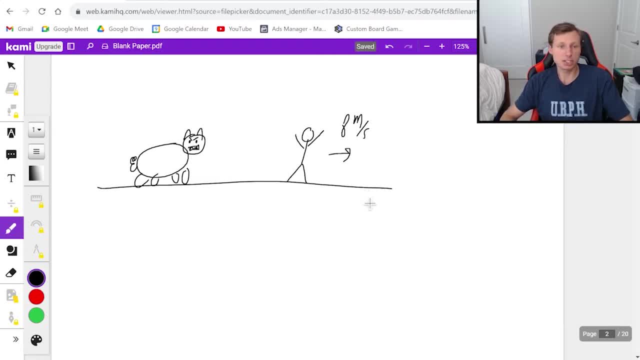 like 16 miles per hour, so you're like sprinting it as fast as you can. And let's say you, the observer, are hearing a frequency of 855 hertz from the bear like it's growling. you hear 855 hertz. 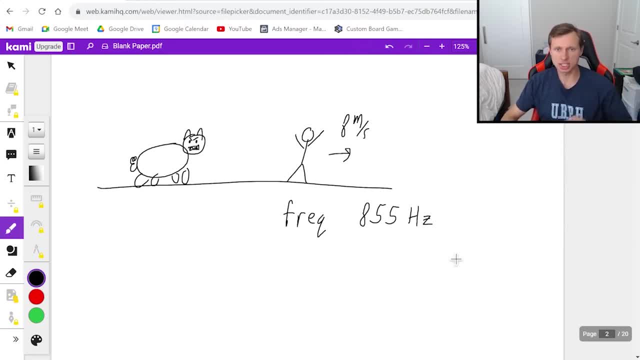 because you are really amazing at distinguishing sounds down to the frequency, But you think, huh, that's strange because, as we all know, the frequency of a bear is actually 850 Hz. In other words, the frequency you hear is different than the frequency of the bear. 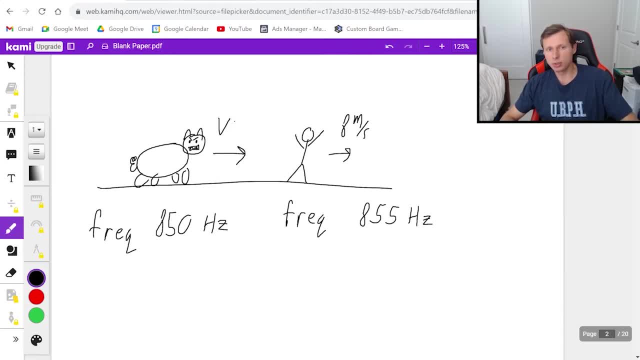 And we all know the reason for that: it's because the bear is chasing you with some velocity. So the question is: in order for this scenario to happen, what is the velocity of the bear? So to answer this question again, we just need to plug in variables into the formula. 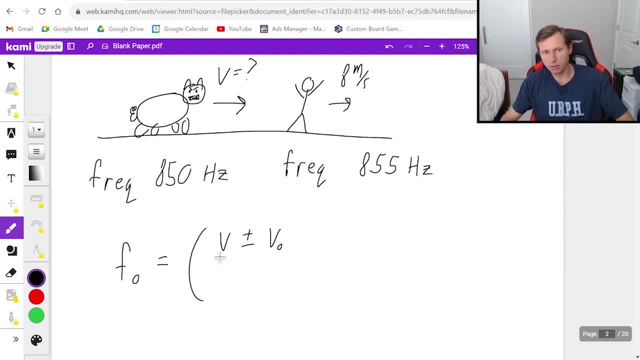 Frequency of the observer equals v plus or minus. vo over v minus plus vs times fs. Looks like the observer u is 855, so I'll plug that in right there. Then the velocity speed of sound that the air is traveling in is 343.. 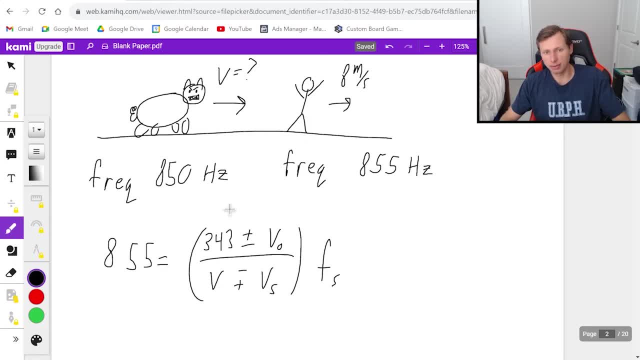 So you, the observer, are you heading towards or away from the bear? Obviously you're running away from the bear. So we should use minus the bottom for the observer, Minus your speed, which we know is 8.. And then in the denominator again, v is 343, because it's the speed of sound and air. 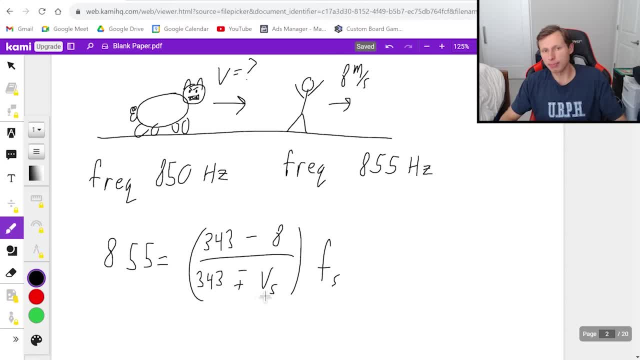 And then I have to think about minus or plus, and that, remember, is for the bear. Now the bear is heading towards us, we should use the top. That one's going to end up being minus as well. We do not know the speed of the bear, so that's what we're solving for. 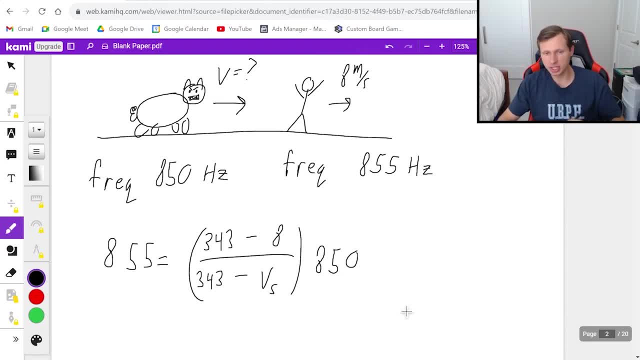 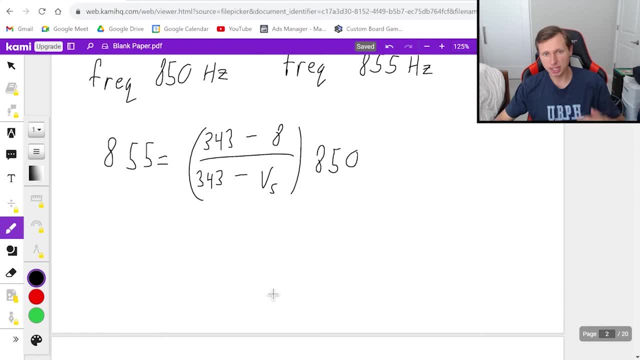 The velocity of the source is 850.. That is the frequency of the bear itself, And now we just have to solve for vs. There's a couple ways you can do this. My recommendation would be very first thing is: divide both sides by 850. 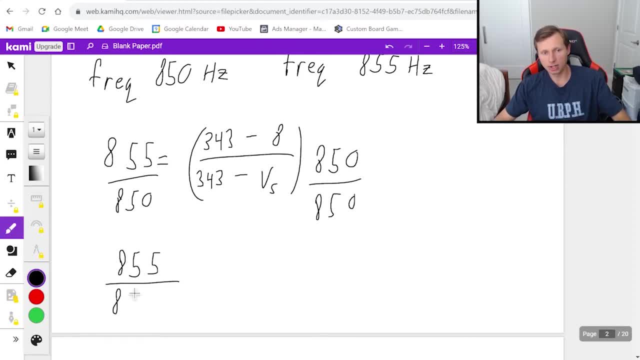 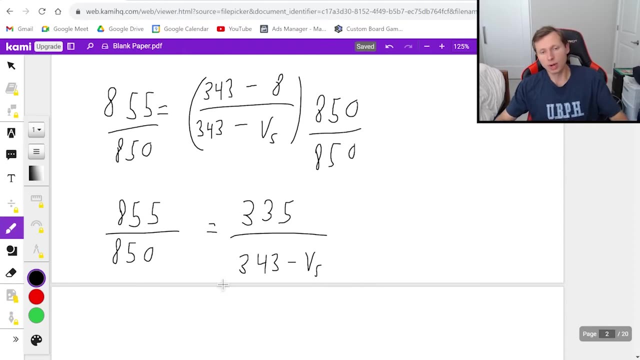 And so now you have on the left 855 over 850.. On the right numerator is 343 minus 8 is 335.. And then in the denominator you have 343 minus vs. Again, there's a couple things you can do here. 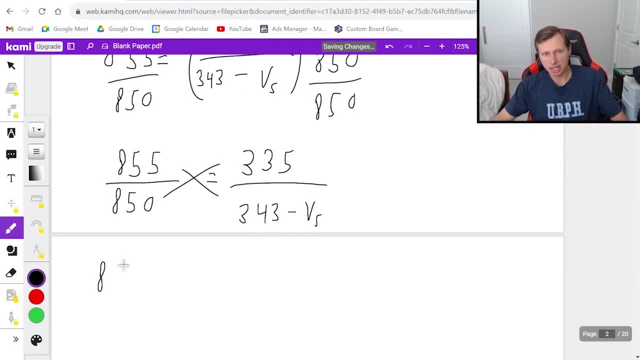 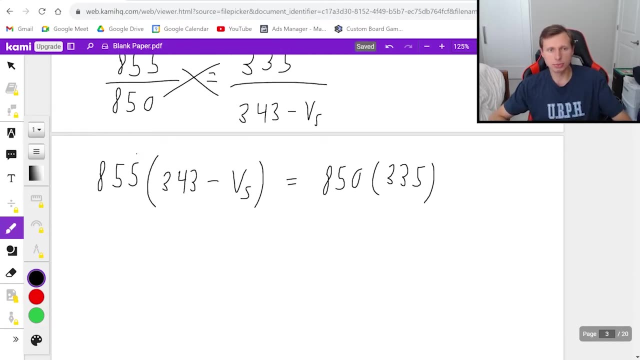 What I would do is I would cross multiply. So on the left, 855 times the quantity 343 minus v of the bear is equal to 850 times 335, which I can plug in my calculator. So first I'll distribute the 855 to both sides here. 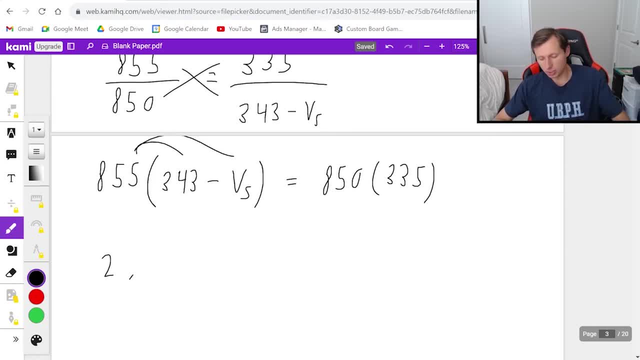 Let's see what's 855 times 343?? Looks like it's a ridiculously big number: 293,243.. 265.. And then minus 855 vs. Hopefully this is making sense. This is like algebra, So if you don't know it, then that's a problem. 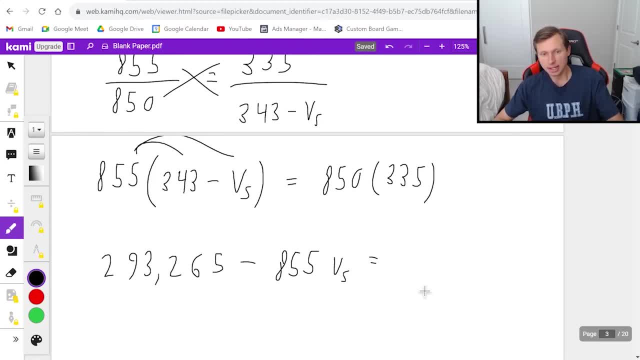 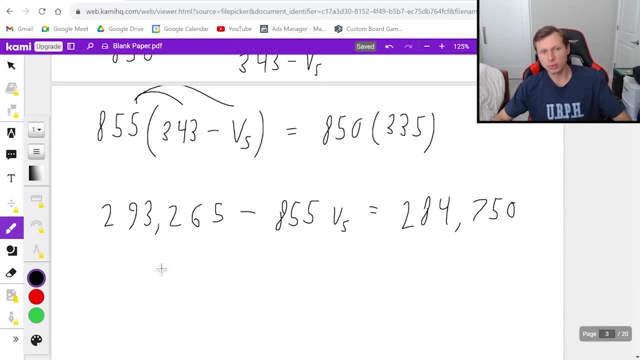 And then the right side: 850 times 335.. That's going to be 284,750.. And finally, if you want to solve for vs, we can subtract this number from both sides. So then we'll get on the left. 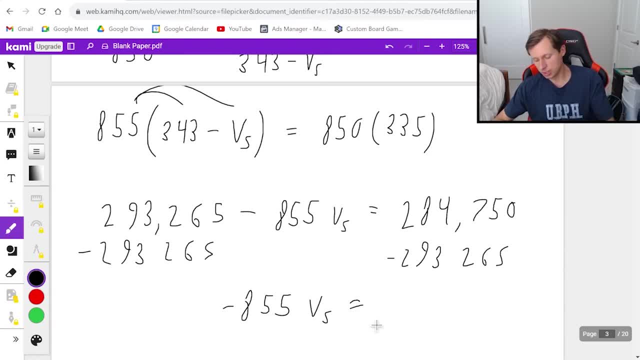 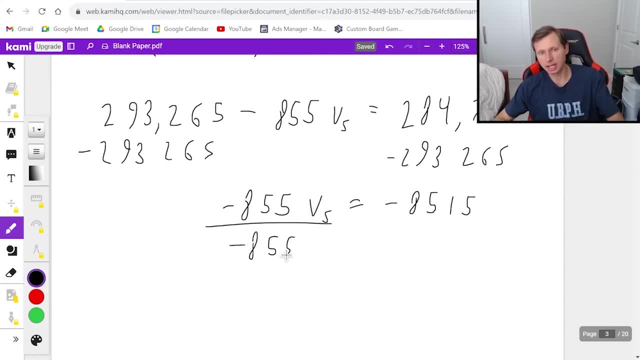 Negative 855 vs equals negative 8,515.. And then we just divide both sides by negative 855. And we'll get a final answer of about 10 meters per second. Not exactly, but it rounds up, And so that's the speed of the bear. 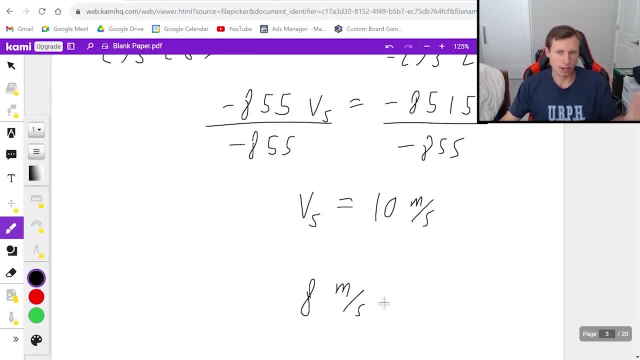 Remember, our speed is 8 meters per second. So basically, we're in trouble And the answer is 10 for this problem. That's the speed of the bear. So once again, you'll notice that the speed of the bear is 8 meters per second. 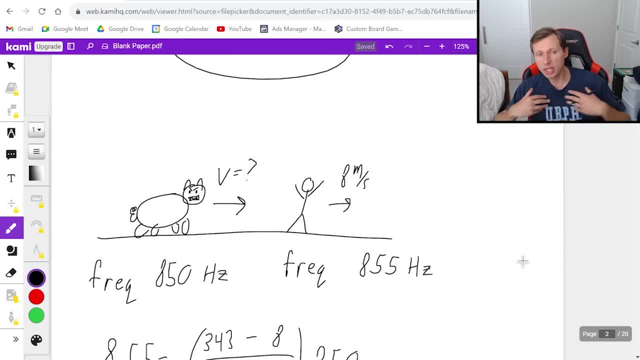 Again, you'll notice that, if I go back to the beginning, the frequency that we hear is going to be slightly higher than the frequency of the actual bear. The reason for that is because the bear is heading towards us. Even though we're running away from it, the bear is still out chasing us. 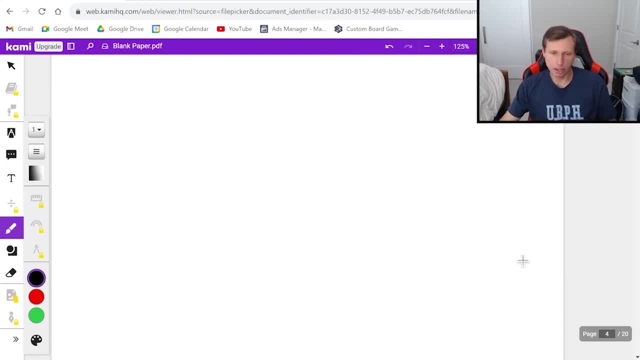 And now we have one more example to do today. This is going to be the echo example. Echo examples are always the trickiest, but the good news is, once you know the secret, they're pretty easy. So let's say we have a train that's heading into a tunnel. 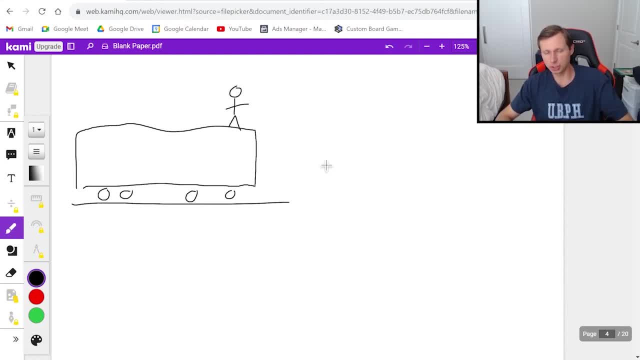 And we're going to be standing on top of the train because we have no fear of danger. And so we're approaching this tunnel right here, very dark, very scary, And the tunnel has a total distance of, we'll say, 1 kilometer. 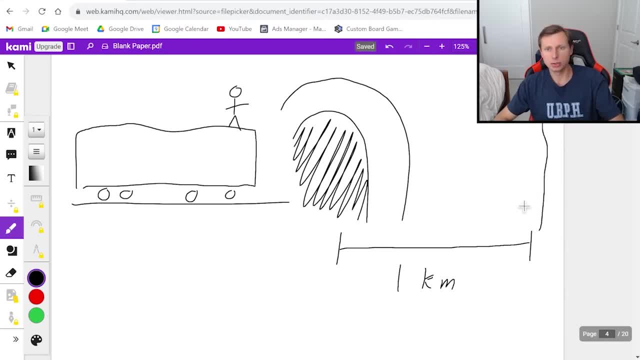 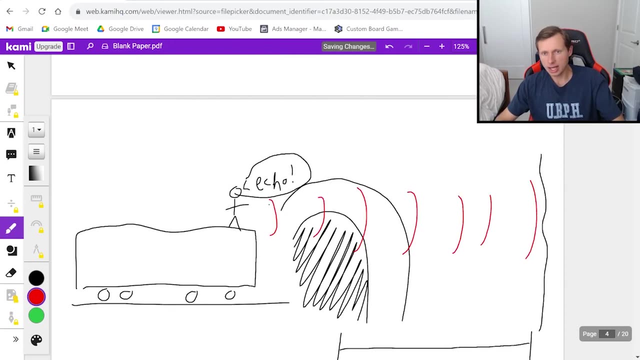 At the end of the 1 kilometer, let's say, there's some sort of wall here that sound can reflect off of, And what you're going to do is you're going to say: echo right here, And then your sound is going to reach the edge of the cave, bounce off of it and then get reflected. 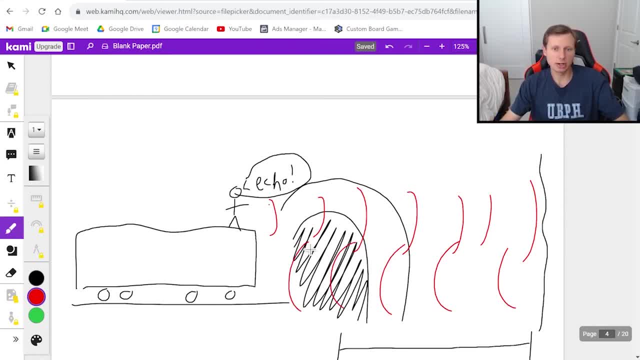 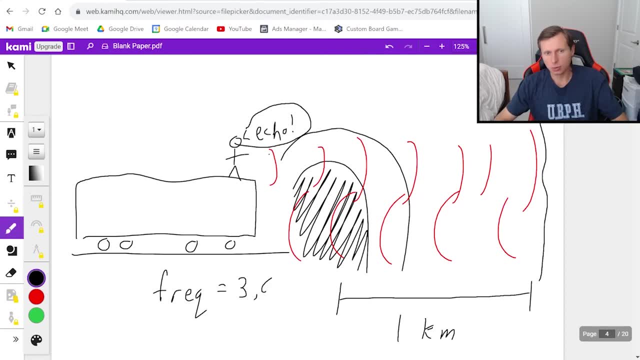 back like this: And then you are going to hear the echo. My question is: let's say your frequency is 3,000 hertz, What frequency do you hear back from the echo? And let's say the speed of the train is moving? 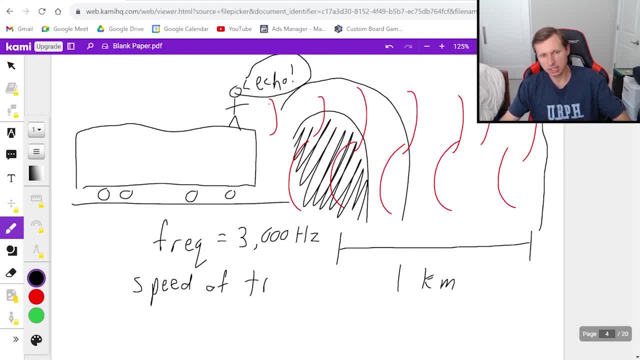 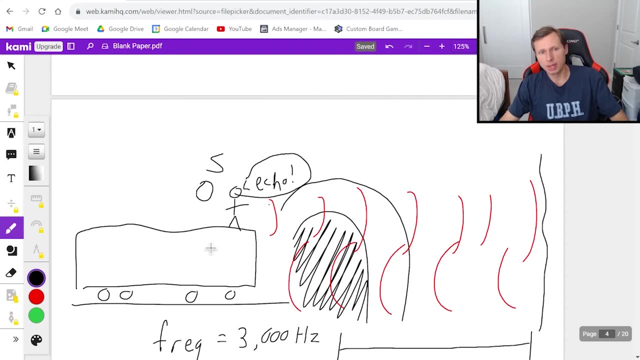 Let's say, My speed of train is 50 meters per second. So the thing about this problem is that it's two parts. The reason why is because you are the source and the observer is also you, But you can't think of it like that. and the reason why is because something weird happens. 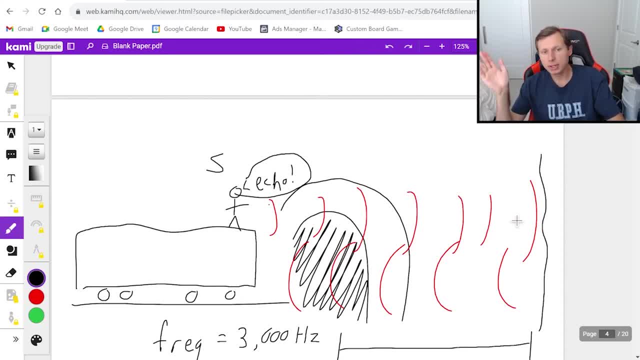 after it bounces off the wall and gets reflected back. So what I recommend doing is split this up into two parts. The first source is you. The first observer is the wall, And then, in the second part of the problem, we're going to make the source the wall and 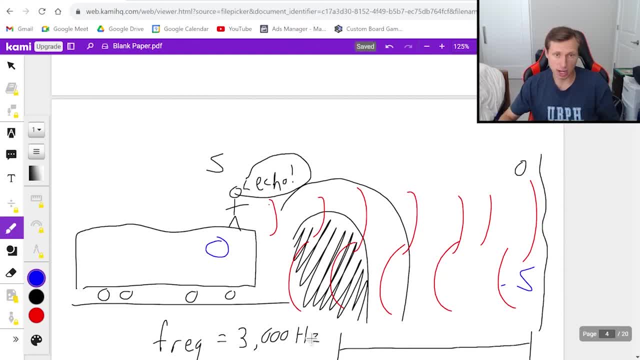 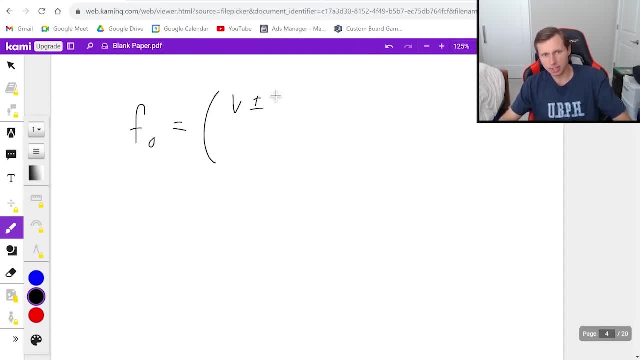 we're going to make you the observer. That's basically how you have to solve this problem. So for the first time, we use the equation fo equals v plus or minus, vo over v minus plus vs times fs. Again, this is for the first part, where the observer is what we're solving for. 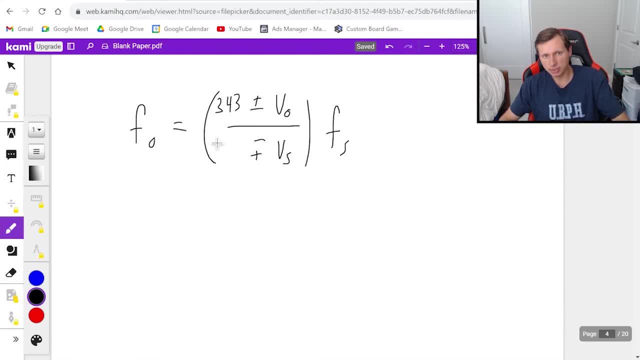 Both of these v's are 343. Because we are sound. So we're going to solve this problem. We're going to use sound in air. The only time you would not use 343 is, for instance, if you're talking about light or 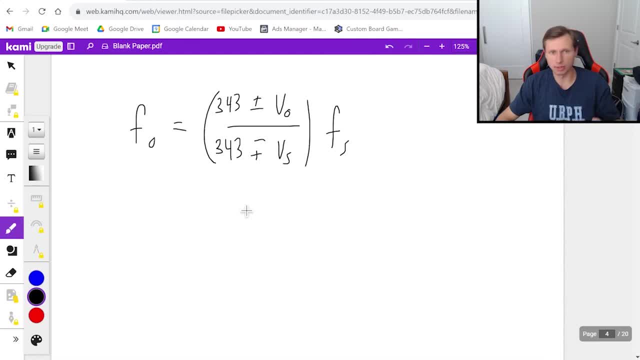 if you're talking about sound moving through water, Then it would be different there too. Then the velocity of the observer. remember, that's the back of the cave wall. Is the back of the cave wall moving? No, That's zero. 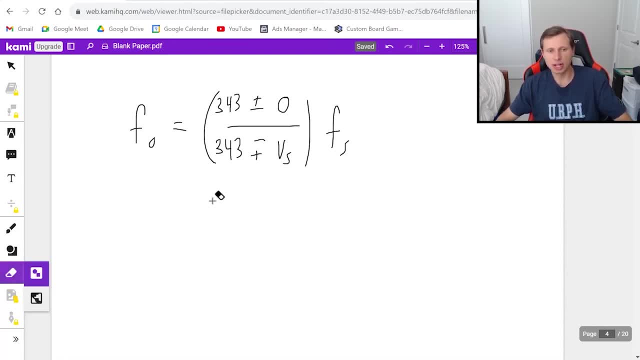 Doesn't matter if it's plus or minus. And then for vs, that's the velocity of us, the source which we're on the train, And the train's moving with a velocity of 50.. And since the train's moving towards the back of the cave, then we're going to use the 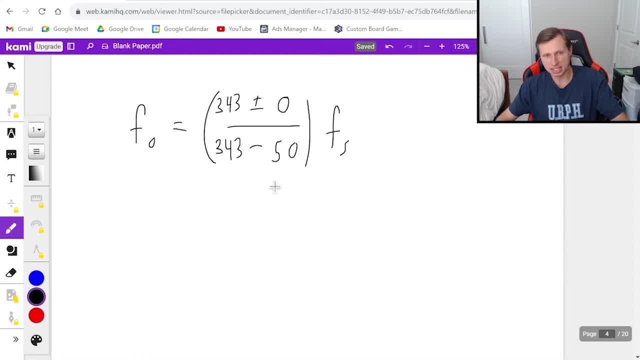 top, because it's heading towards and the top is minus. And then times fs, which our source was 3000 hertz, And so now I can just plug this all in a calculator and see what the observed frequency is. It looks like I get an observed frequency of 3512 hertz. 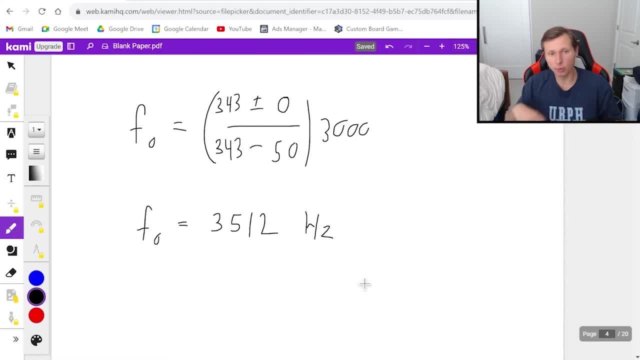 Again, this is not the final answer. This is just at the cave wall. We still need to do this equation a second time to see what the actual observed frequency is back on the train. However, before I do that, I just want to make a little prediction. 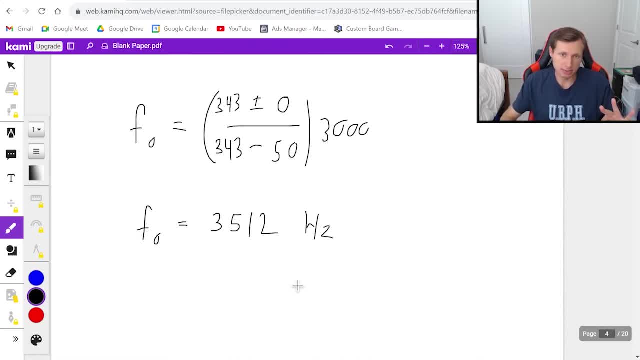 My prediction and just so you know, I did not do this problem ahead of time, but my prediction is that the answer is going to be 4024 hertz about. That's my prediction. Let's see if I'm right. 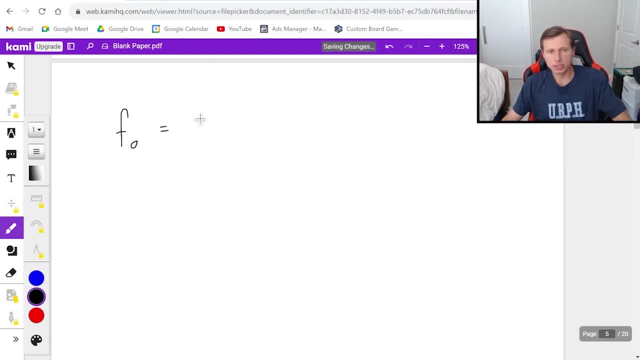 So what I'm going to do is I basically do the same equation. frequency of the observer equals, The denominator is 343, plus or minus. The cave wall is now the source. so we, the people on the train, are the observer. 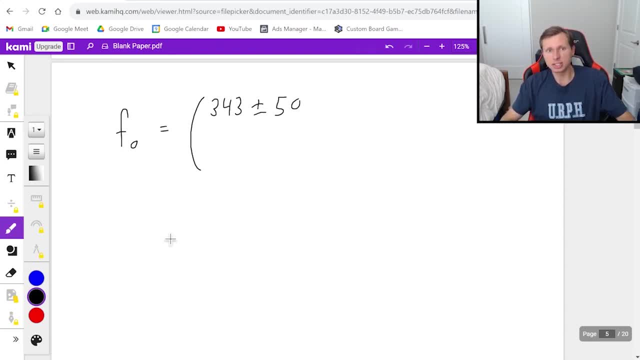 What I'm saying is that, since we're the observer, now that's 50. And since we're heading towards the wall, we need to use the top because we're heading towards, so plus, And then the denominator is 343 minus plus the source, which is the wall. 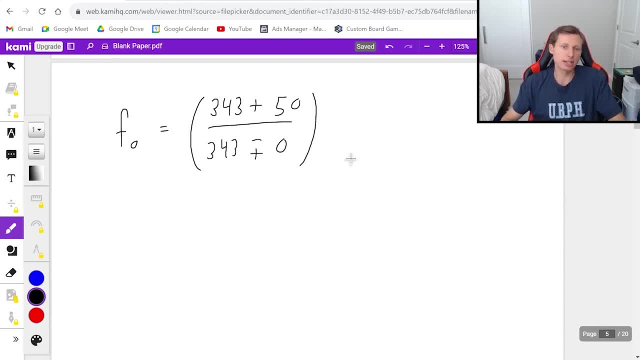 Again, the wall is not moving, so zero. And then finally times the frequency of the source Again. So the second half of the problem: the source is the wall, which is the answer we just got a second ago. It was the 3512 number from the first equation. 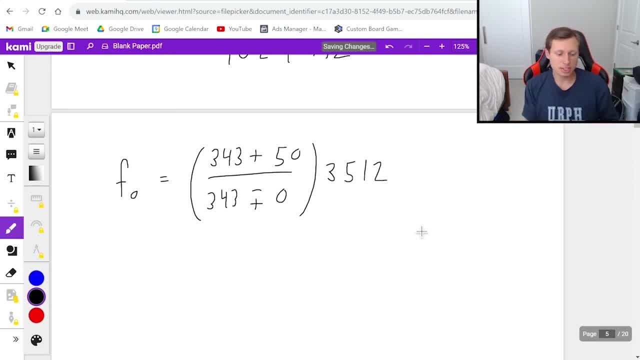 So times 3512.. Again, I plug this in a calculator and it looks like I get a final answer of 4024 hertz, Which is funny, right, Because that was my prediction before I even did the equation. Now, of course, the question is: how on earth did I know that? 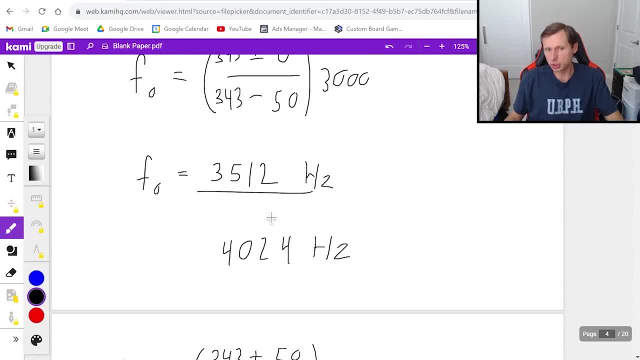 So basically, I look at the answer I got for the first part, Which was 3512.. And let's subtract that from the original frequency to find the difference. In other words, the difference for the first half was an increase of 512 hertz from the. 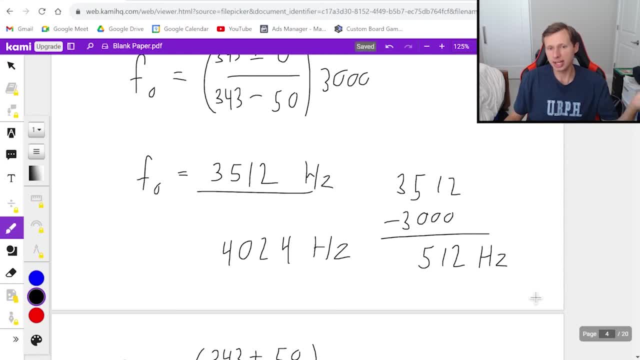 first half. Since this is symmetrical, I just knew that the second half was going to be another increase in 512.. And 3512 plus 512.. That got me this, And I did that in my head because it wasn't that hard to do. 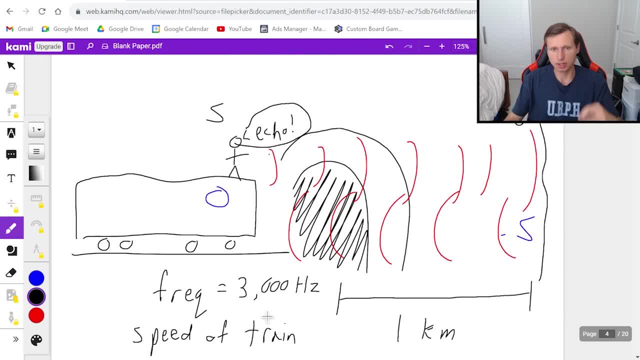 So, in other words, we just discovered a second way to do the cave example. First, Find the observed frequency at the wall, Find the difference or the increase- in this case it was an increase of 512.. And then just double the increase.